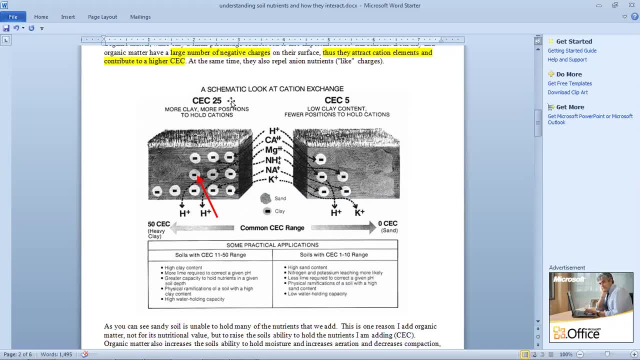 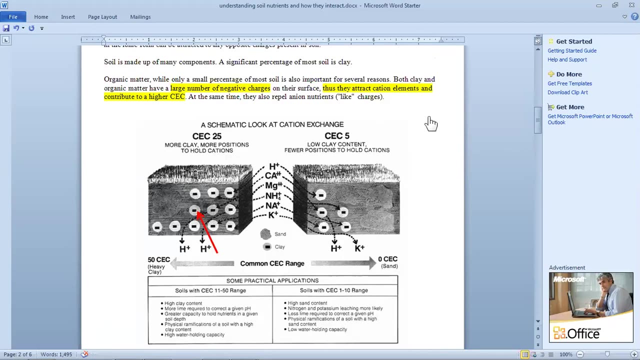 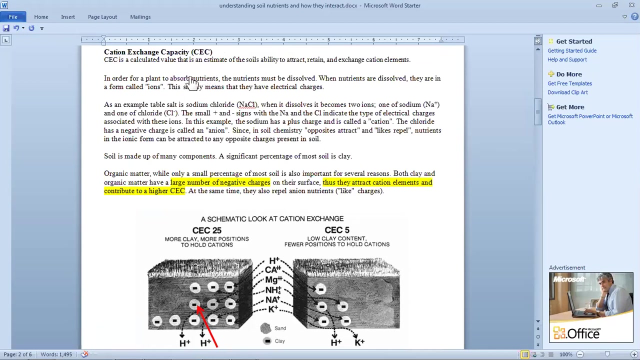 positive ions. the more CEC you have, the more your capacity in your soil to hold on to nutrients. the sandier your soil, the lower capacity you have. so if you have, as we read this, in order for your soil to absorb nutrients, the nutrients must be dissolved, the nutrients whenever they're. 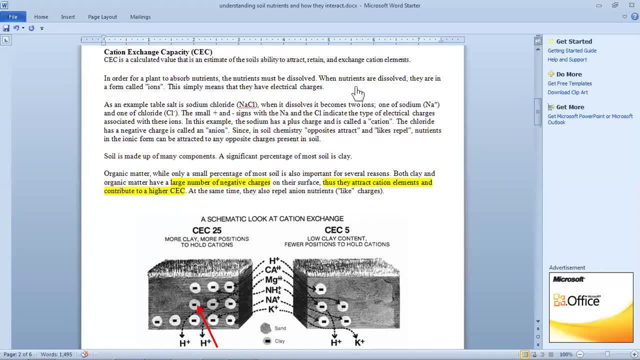 dissolved. there they become ions, which means that they're charged. and then it gives an example here of sodium chloride. there's a positive sodium atom ion and a negative chloride ion, and in this example the sodium is positive. it's called a cat ion, which is what the CEC is called. is the cat ion. 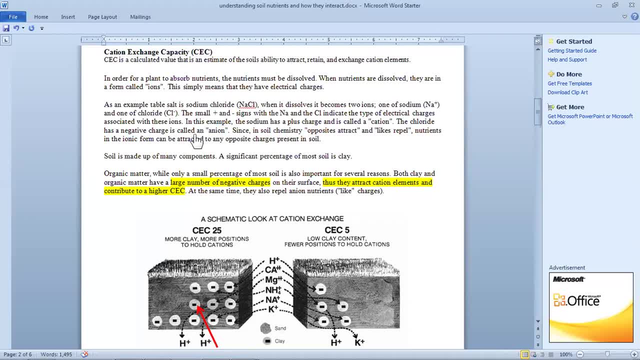 extractor and the chloride is a negative charge which is an anion and it's an. it's an opposite. opposites attract to each other's and likes of a repel. that's important and we'll talk about that quite a bit tonight. nutrients in the ionic form can be attracted to any opposite charge present in the soil. 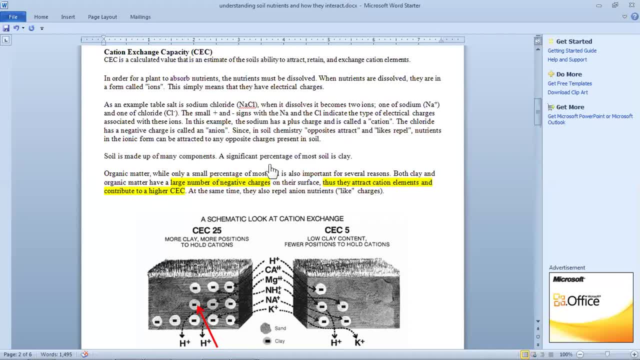 soils made up of many components, and the significant percentage of most soil is clay. there is portions of our growing that have a lot more sand, so ideally you would want something that have higher CEC in order to be able to contain the nutrients that we need. you can add organic matter, and it usually in normal 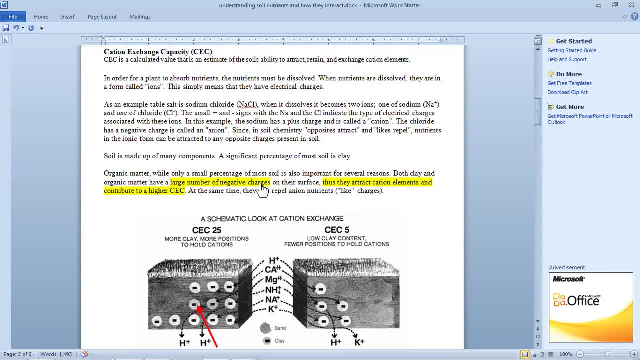 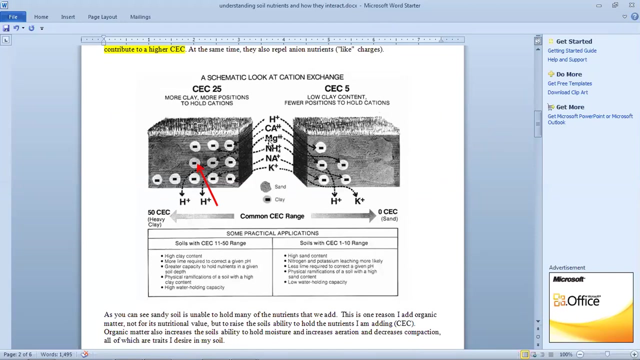 soils. it's a very low percentage, sometimes as low as two percent of that um. both by adding organic matter and clay you can raise your cec and at the same time that that will repel anions. so this gives some examples of calcium is a plus. 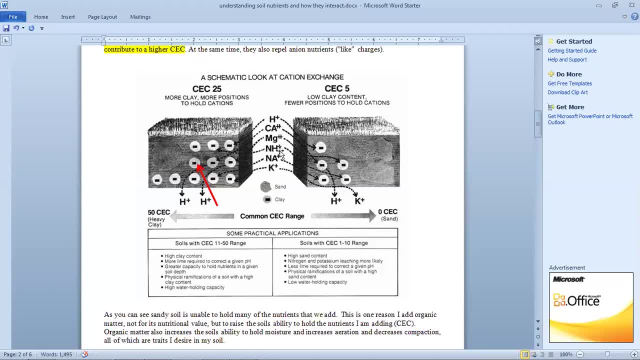 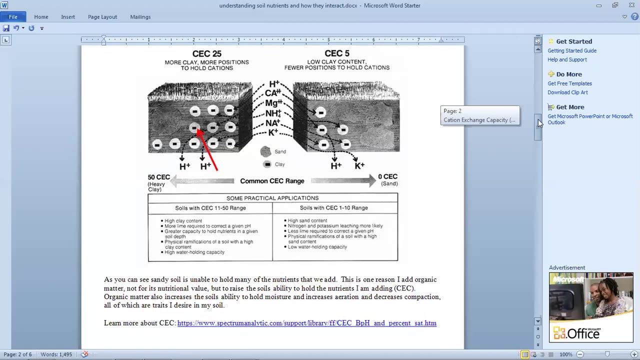 magnesium is a plus, nh is uh- ammonia, i believe- and n, a is salt and k is potassium. and, as you can see, the sandy soil is unable to hold many of the nutrients that we add. this is the reason that i add organic matter, not necessarily for nutrition, but to raise the soil's ability to hold the nutrients. 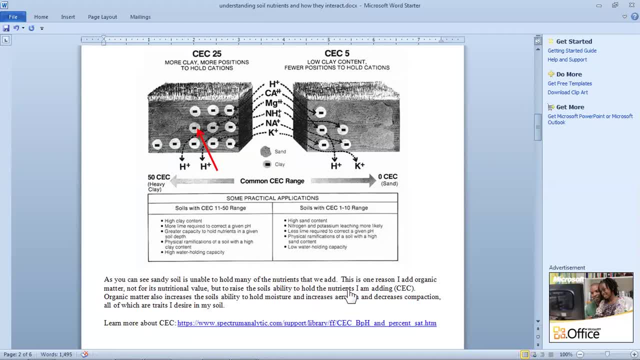 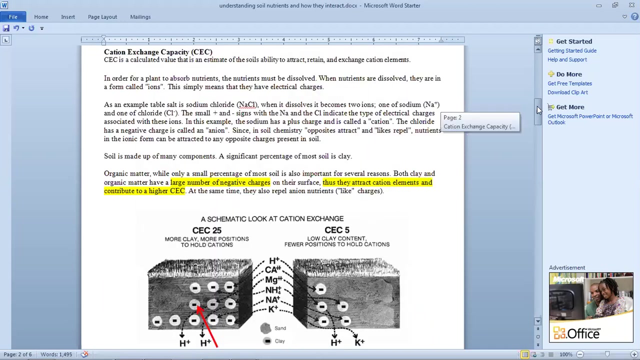 i'm adding and raise my cec, so that's the reason why i'm adding organic matter. organic matter also increases the soil's ability to hold the moisture and increases aeration and decreases compaction, all of which are traits that i desire, and i got this clip and a lot of this, these words from spectrum analytics. they have a wonderful 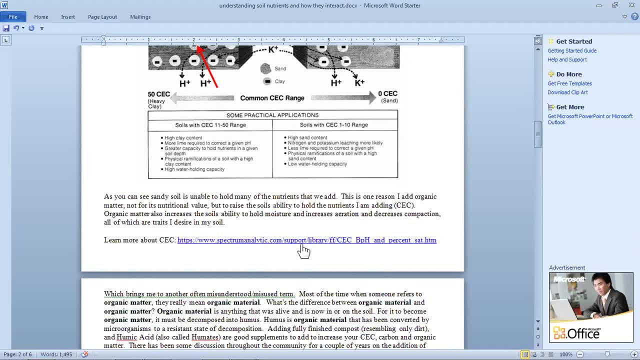 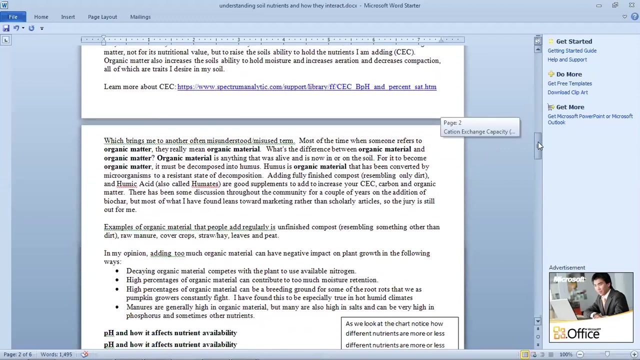 library about all kinds of things growing. i suggest everybody go to the their library and browse and read and read and read. you will learn a lot of things from this and it's and it's in. there is scientific stuff, but it's in understandable terminologies. so we've talked about organic matter a lot of times. people will say something is or 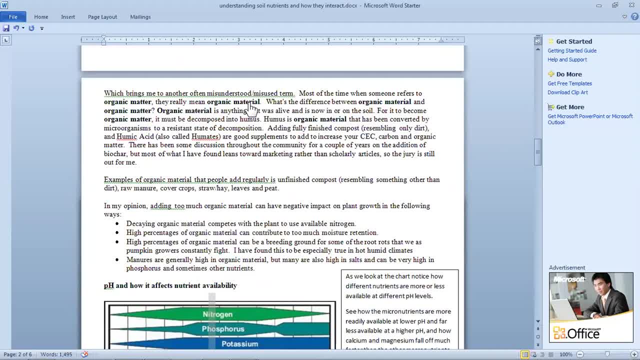 they're adding organic matter, but they're really adding organic material. what's the difference between organic material, organic matter? organic material is anything that was alive and is now or on in or on the soil, for before it can become organic matter, it must be completely decomposed and turned into humus. humus is organic matter that has been converted into micro. 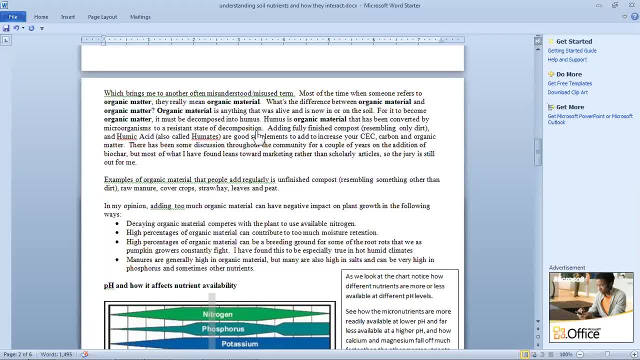 by microorganisms into a resistant state of decomposition. so, basically, if it resembles anything besides dirt, it is organic material. it's not organic matter. and if you add- i add humic acid every year, which is also called humates- there are different levels, different grades, if you will, of humic acid. 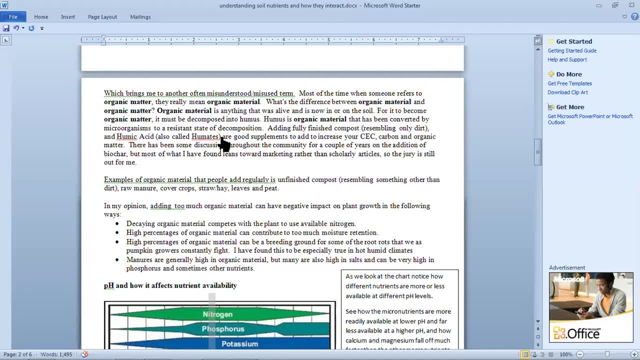 and it's going to be a different kind of acid. you can call it humic acid and it's going to be humic acid and it will be humic acid and coenomal acid and all different kinds of humic acid and coenomal acids you can use. through your plant. We have had lots of discussions over the last probably five or six years about adding biochar. I really haven't found any studies that I thought made a difference. It's kind of expensive and I believe a lot of people are trying to make their own. The way that it's created is by burning without. 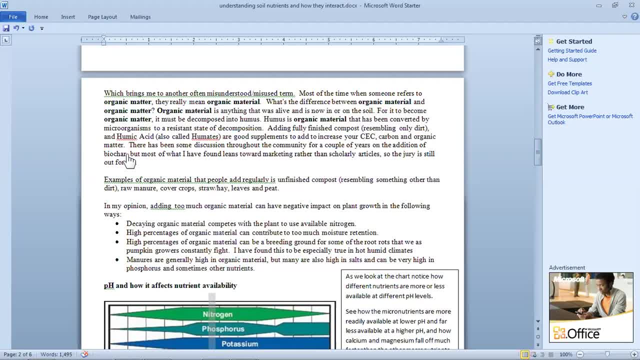 oxygen. So to create your own. I don't know if you could really totally and completely emulate how it should be made in order to be beneficial. So and then I give some examples of organic material which would be unfinished compost, presumably something other than dirt. raw manure, cover crops, straw, hay leaves, peat. These are things that everybody adds. I add them, But if you add too much you can get a negative impact on your plant growth because of these conditions. The decaying matter competes with the plants. use of available nitrogen. In order for that organic material to decay it has to use nitrogen And it will use the nitrogen and your plant won't have enough Now as the cycle continues. it'll become more available as it breaks down the organic material. So if you have enough nitrogen, then it's not necessarily a bad thing. But I've seen people over and over and over again add way too much organic material and their plants suffer because they don't have enough nitrogen. You need to add more. If you're not getting good plant growth, especially if you have high organics that you're adding. I've also seen people that whenever they add too much, it gets too wet, And when it gets too wet you usually get a anaerobic situation where it starts smelling it's decaying but it's not. getting enough air And that's causing, In my opinion, the stink is bad, You're getting the negative, the bad microorganisms are generating and getting too many of them in your patch and they can cause you problems. The other thing I see a lot of people doing- 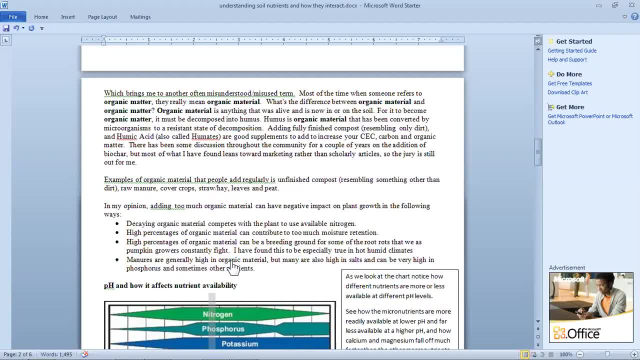 is adding manure. If you add manure, it can have a lot of organic material in it, but it's also typically very high in salts in urea And it can be very high in phosphorus and sometimes other things too, like potassium. 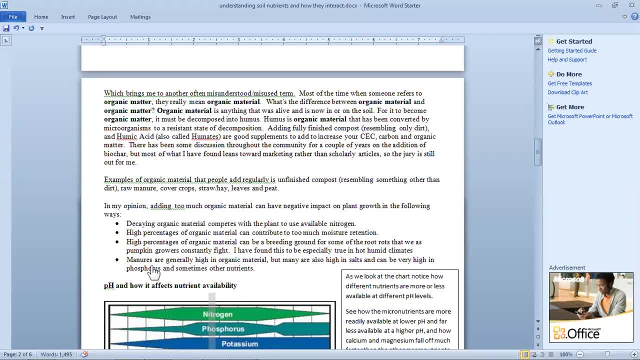 If your phosphorus gets too high, it takes years to lower it. It doesn't move in soil. It's something that I try to when I'm helping people understand their soil. you gotta back off on the phosphorus because if the phosphorus is too high, you're locking things up And we'll talk about that a little bit later. So now we'll go into how pH affects nutrient availability. The pumpkins will grow anywhere from about 5.5 to 5.5 to somewhere close to eight. But you don't just wanna grow them, You want them to thrive. And if you get the pH somewhere between 6.5 and seven, that's the band- if you look where almost it's the perfect band- of where all of the nutrients. are the most available. You'll see, as the the pH goes down, magnesium's less available, calcium's less available. As the pH goes up, all of your micronutrients, except for molybdenum, are less available. the higher the pH you go. So typically I try to target between 6.8 and 6.9.. But pH is kind of like one of those things that if your soil is naturally, whatever your soil naturally pH is, it's gonna try to rebound to that. So you just it takes a long time to actually get it to change and stay. So it's not a one time put some lime on or one time put some sulfur in. If your pH is normally- and I've seen it. 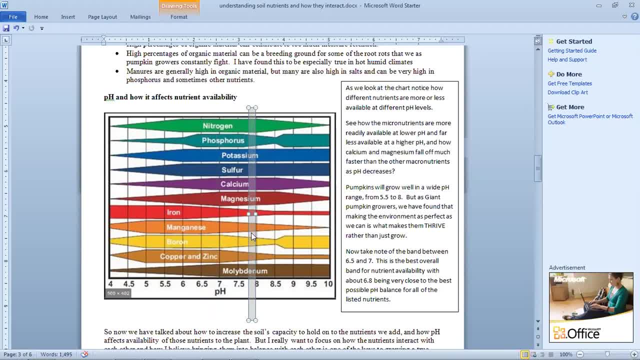 way up here by eight. you may never get it below seven. So you just gotta learn your soil and how it's available. And if you've got a pH of eight, you may have to add micronutrients through the year, And you just have to know that. There's a lot of really, really great growers that target 7.5, because at the higher pHs a lot of the diseases can't thrive. So what they do is they target 7.5 and they supply micronutrients. There's absolutely nothing wrong with that way of growing. 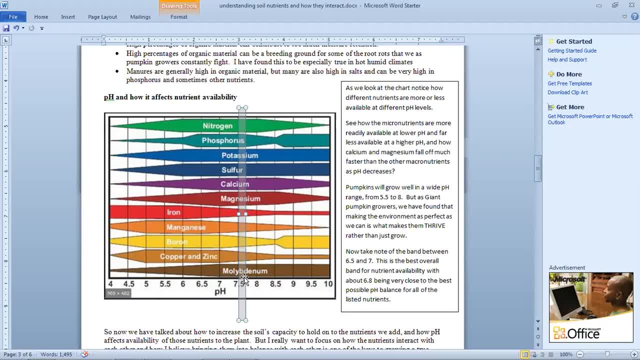 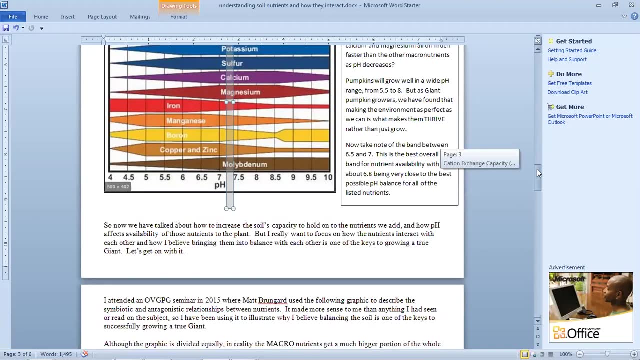 as long as you know that you have to supply these micronutrients continually Because they're not gonna be available at a higher pH. So that's the availability of pH. So we've talked about how to increase the soil's capacity to hold nutrients. 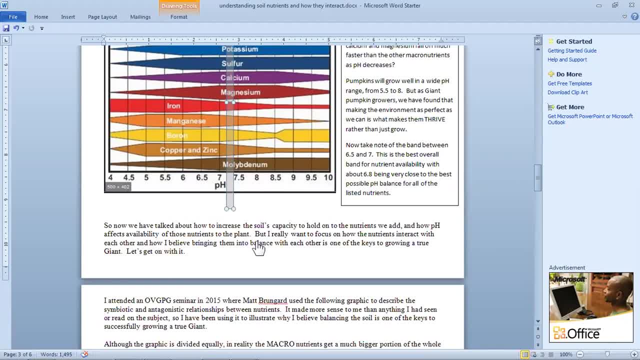 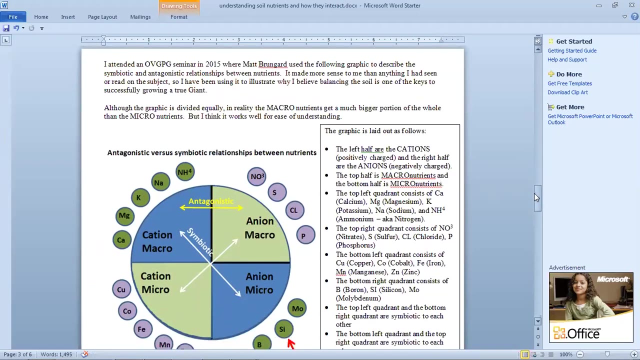 and how pH affects the availability of the nutrients. But I really wanted this presentation to focus on is how they interact and why I believe that balancing them out is the key to growing giant pumpkins. So I attended a OBGPG seminar in 2015,. 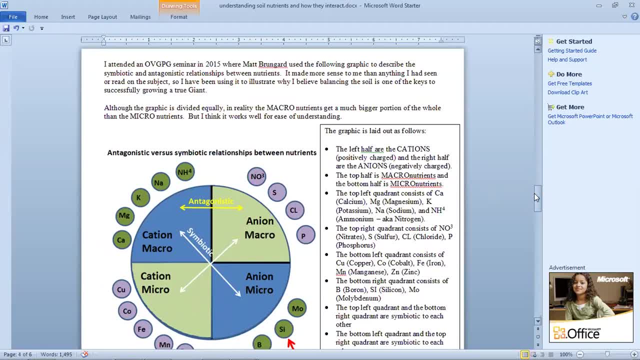 where Mike Brungard had just grown a 1900 plus pound pumpkin And he did a lot of study on soil. And I was studying soil at the time, trying to understand it, trying to wrap my head around it. And I was trying to understand it, trying to wrap my head around it. 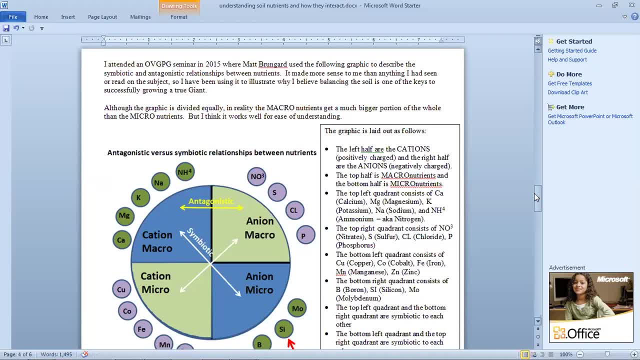 And I had used the soil calculator a couple of times and it worked, but I wasn't really. I mean, I had read a lot of things and I wasn't really wrapping my head around how the nutrients. I was just taking what was written down and saying: 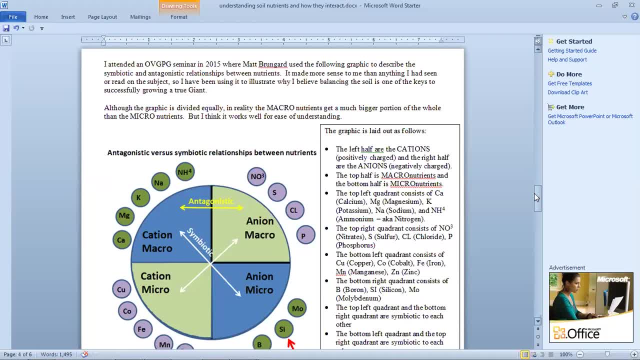 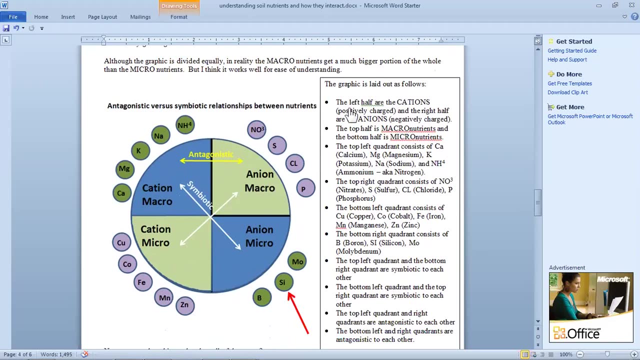 well, these ratios are what I have to strive for, But I didn't really know why. So, whatever he showed us this chart, it made the most sense to me and it actually clicked. So to describe the chart, I've got a whole list of things over here on the right. 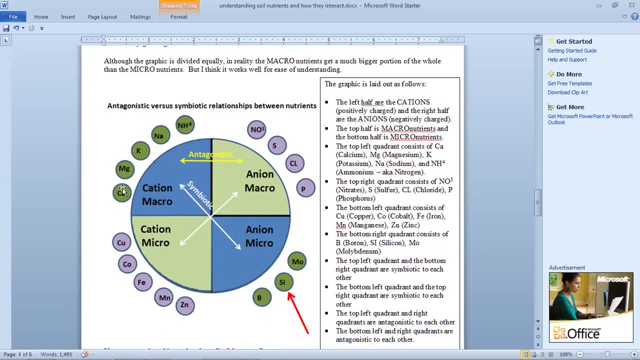 The left half of this chart. So all of these nutrients are all your cat ions, All your positive charged nutrients, alright, and the top portion is your macronutrients and the bottom portion are your micronutrients. and that goes this way, too, on your anions. this whole right side is your anions. 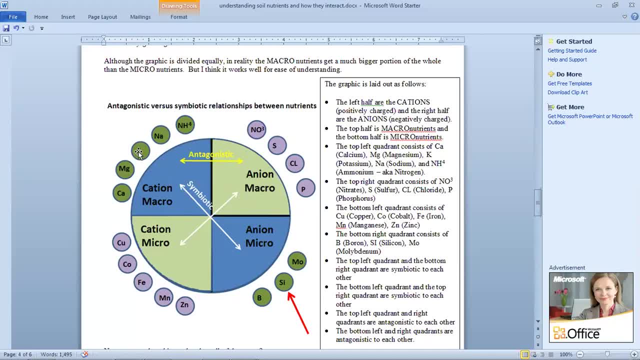 so, in order for the interactions between, the symbiotic interactions between your cat ion macros and your anion micros work together, and the same thing for your cat ion micros work together with your anion macros. so, and if side to side, because this is the positive, 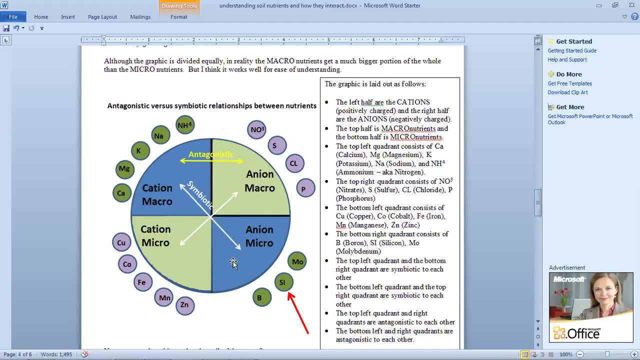 side, and this is the negative side- they work against each other. so this particular chart really really kind of drug it home to me is if i knew that i needed the calcium and the boron to be in sync with each other, but this made it click. i was like: oh, and the same thing with the boron in the, in the potassium. 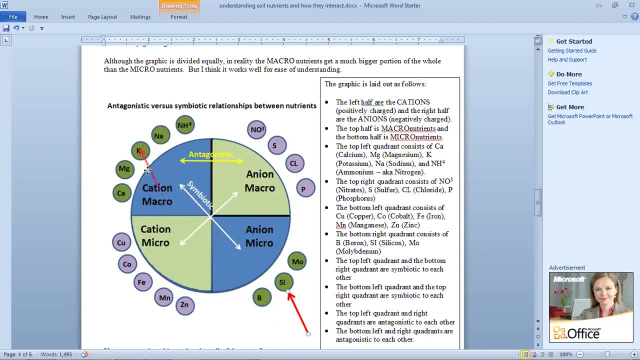 those work together and if those are not in sync then you won't get the best out of what you're doing. so, looking at the chart, and just i i even put over here on the chart, in case people don't know what the uh, the scientific uh- abbreviation for each one of the nutrients is, i put it over here: 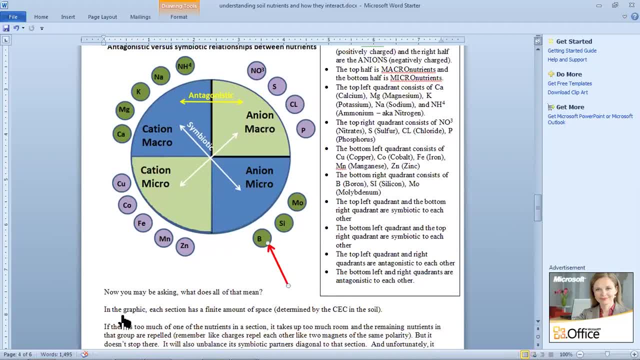 so, to put it all together, there's a finite amount of space in your cec. there's only so much stuff that can happen that you can hold on to. you could put down 10 000 pounds of something. if your soul can only hold on to a thousand pounds of it. the rest of it is going to be washed away or it's going to tie to. 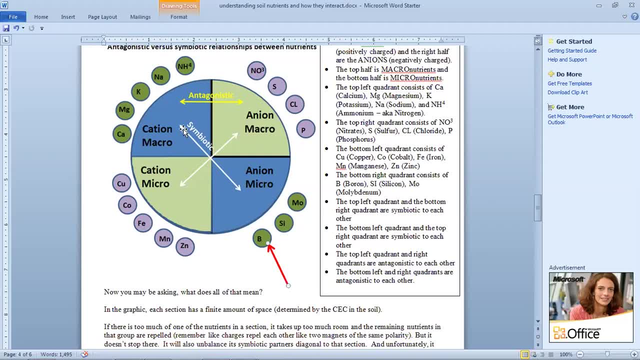 each other because of the positive and negative. so like, if you put down, you know, 10 000 pounds of calcium, it's got a positive, it's got a negative charge because it's no, it's got a positive charge because it's drawn to the cation, which is negatively charged. 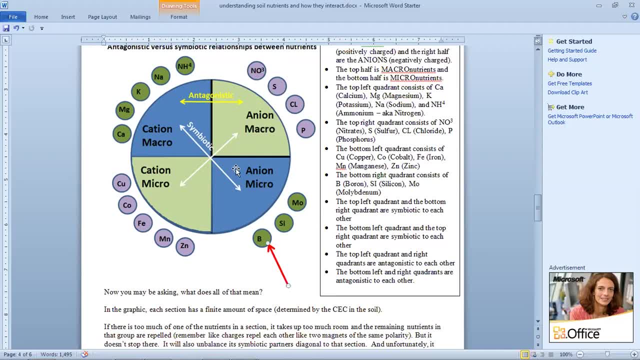 but all of these things over here also have negative charges, so they'll tie to each other. so the calcium will lock up all of your nitrogen, all of your sulfur, all of your chloride, all of your boron, all of your silicon, all of your lipid, because there's so much of it, and the way that the electrical charges. 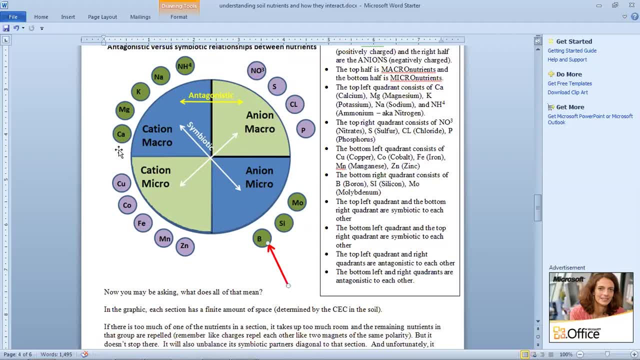 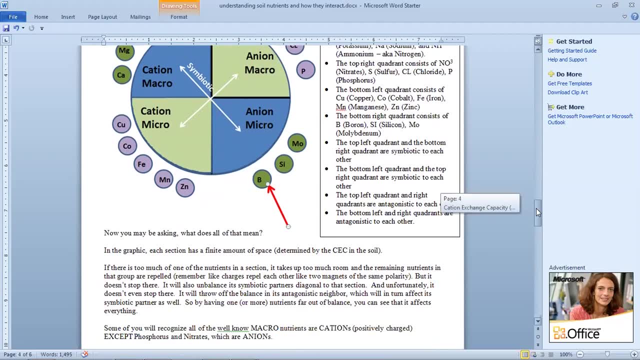 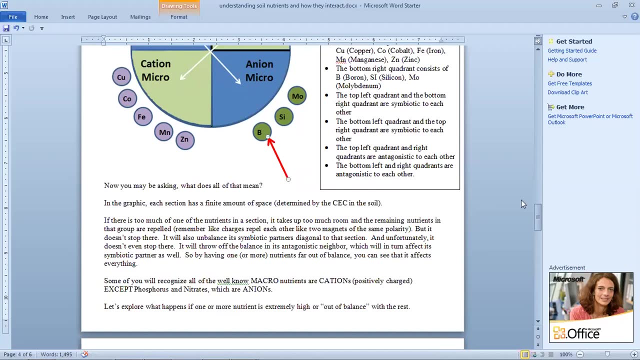 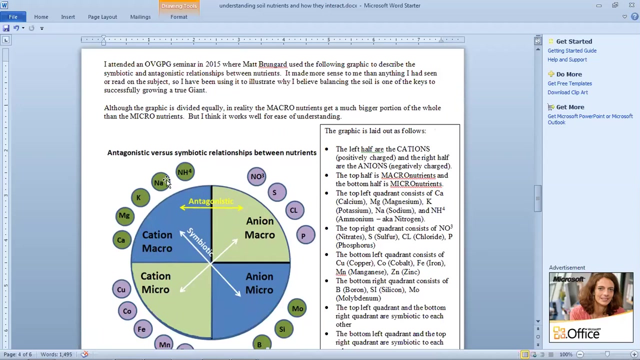 tie to each other, they bond and then they don't. you can't use them. so i made an example down here is: if there's too much of one nutrient in a section, it takes up too much room in that section, so you can only fit so much: calcium, magnesium, potassium. 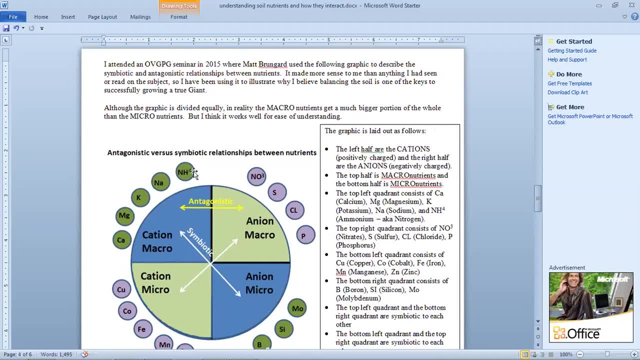 salts. believe it or not, you need salt and ammonia in this section. now the section shows that it's the same size on all of these, and they're not. the micros are smaller. but in order to kind of make it easier to understand, it seemed like it was. 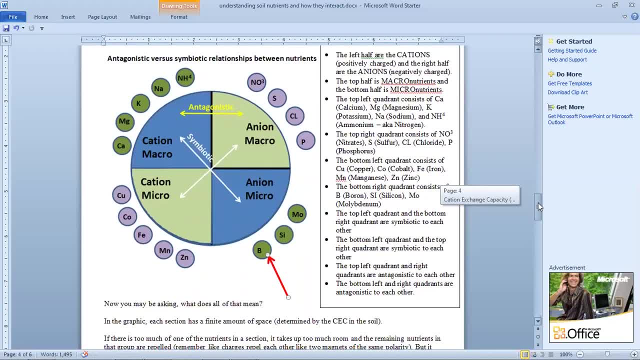 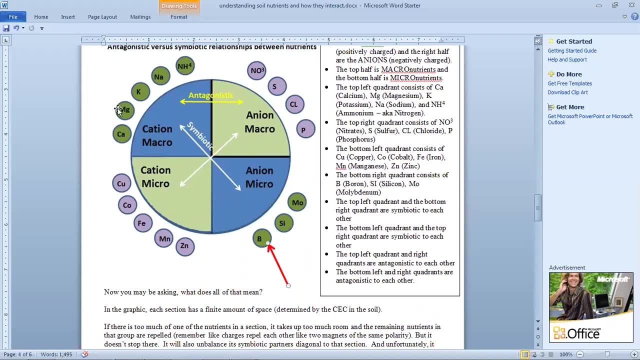 the best way to do it is just make it like a pie, um. but here, regardless of that is, there's still a finite amount of ability of your soil to hold on to things and if you get them balanced and you get the right amount key to each other in the ratios. 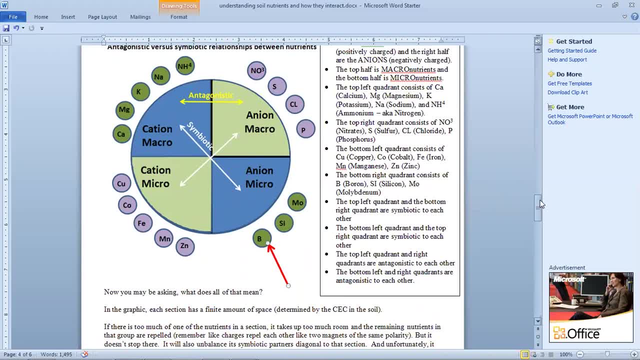 then i think using the soil calculator i have helped more than a hundred growers best, their personal best, by as much of their energy as their выступing potential shares. so if you're using your soil calculator and you need ablok, then know to use out it. much as six to seven hundred pounds simply by balancing their soil. some growers that had been growing for 20 plus years that were great growers. the first time they used the soil the output from the soil calculator went from 1600 pound pumpkins to 1900 pound pumpkins, and that was all they. changed. so- and i i'm one of them- i went from a 1300 pound pumpkin to a 1700 pound pumpkin the first year i used it, and then i was like whoa, and the next year i used it i went. i went from 1700 pounds to 1900 pounds. so i really believe that balancing the soil is the difference.